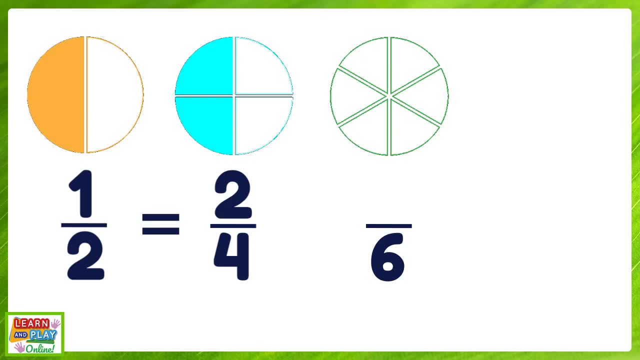 How many parts would we need to shade to make it equivalent to one, half or two quarters? We would need to shade three parts. That's right. If we shade three parts, that would make it equivalent to one half as well as two quarters. 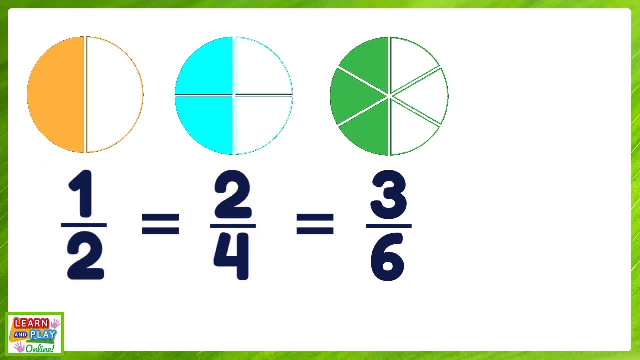 because they all represent the same amount shaded. Let's try one more example using the same circle, but this time we are going to have eight equal parts. If there are eight equal parts altogether, that means the denominator is eight To find the equivalent fraction as the fractions before, how many parts do we need to shade? 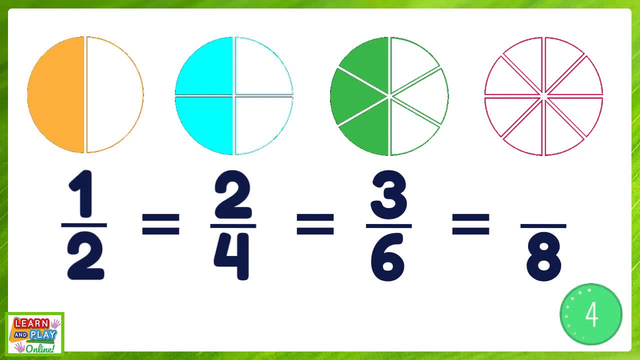 in this new circle of eighths, We would need to shade four parts. We would need to shade four parts. Well done, Four eighths is the equivalent fraction to all of the previous fractions we've looked at, because they all show the same amount. 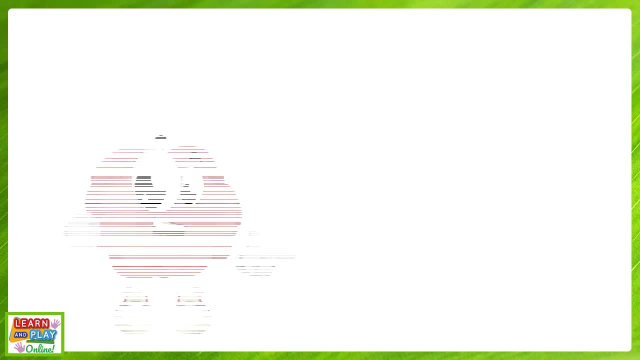 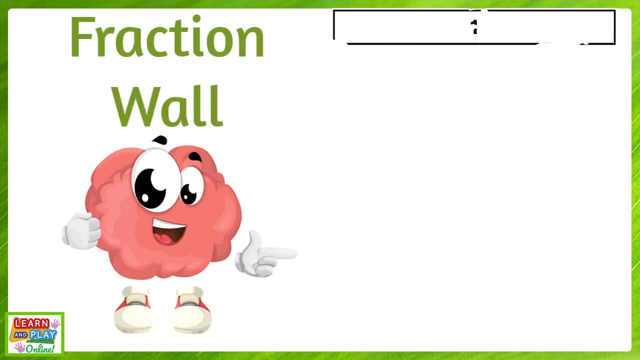 There are other ways we can identify and represent equivalent fractions. One of the easiest ways is with a resource called a fraction wall. Here we have a whole rectangle. We're going to create equal parts with this rectangle, as we did with the circle. 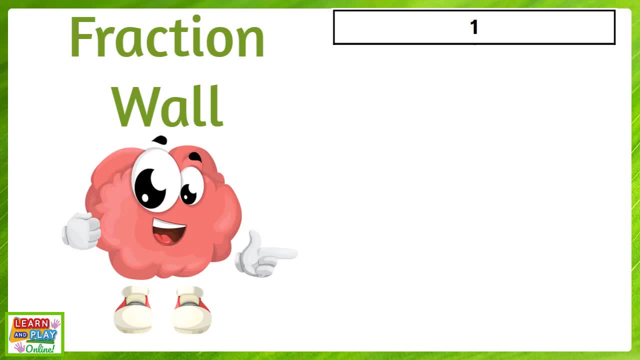 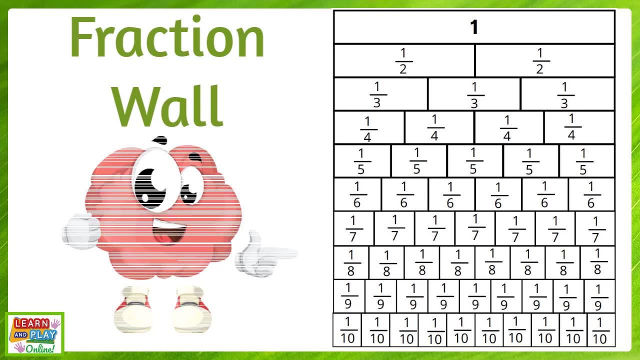 We are going to create equal parts with this rectangle, as we did with the circles. We can create two equal parts, three equal parts, four equal parts, and so on. When we looked at equivalent fractions using the circles, we discovered that one half is. 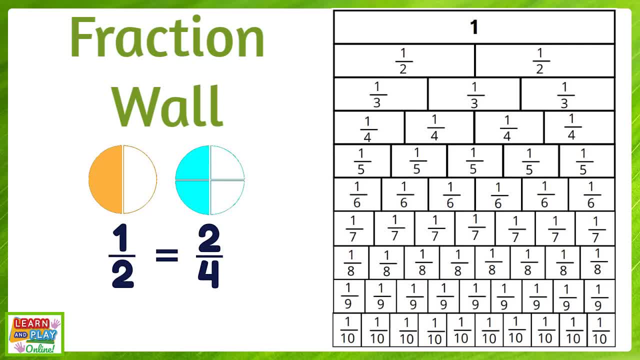 the same as two quarters. Let's see if that is true on this fraction wall too. Here is one half, Here is one quarter and two quarters. As you can see, they both show the same amount. Looking at the fraction wall, can you see the next fraction that is equivalent to one? 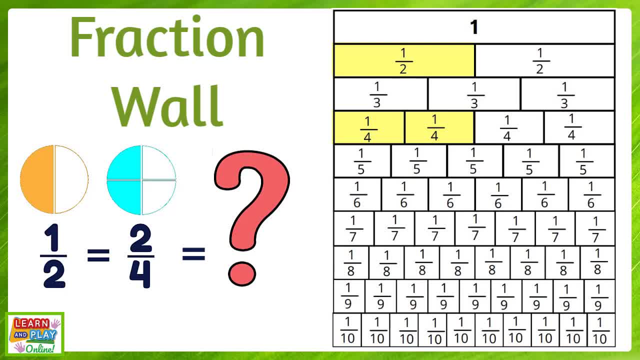 half or two quarters. If you said three sixths, you would be correct. There are another two equivalent fractions to these ones on the fraction wall. Can you see what they are? OK, Let's take a look. The other two equivalent fractions are four eighths and five tenths.